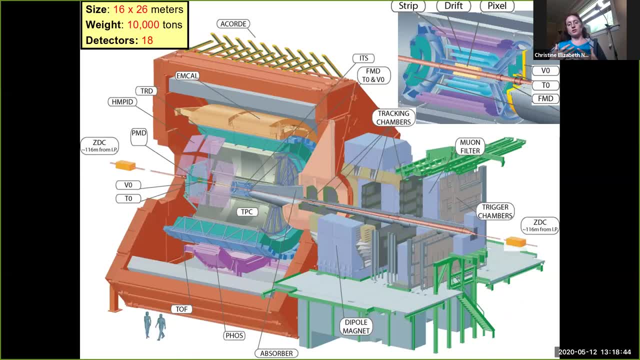 think about the main purpose of these detectors as primarily acting as a camera taking pictures of the particles coming out from the collision. So you need to know the differences that you have depending on the accelerator and the year and so on. You have collisions happening typically about a thousand times a second. It is really fast. So 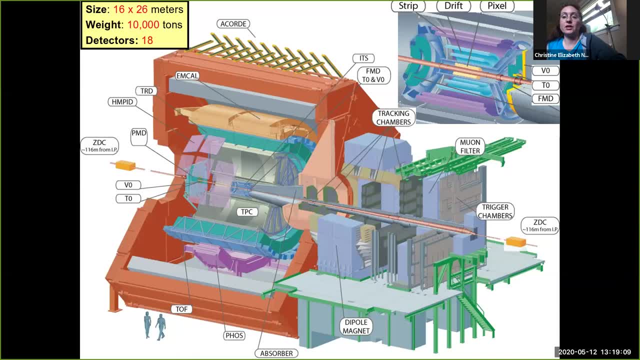 when you can't sit there and tell your detector when to start recording data. so you have one class of detectors that are trigger detectors that tell you when you have a collision, so when you should start recording data. There is one more, another set of detectors that are tracking detectors that tell you where 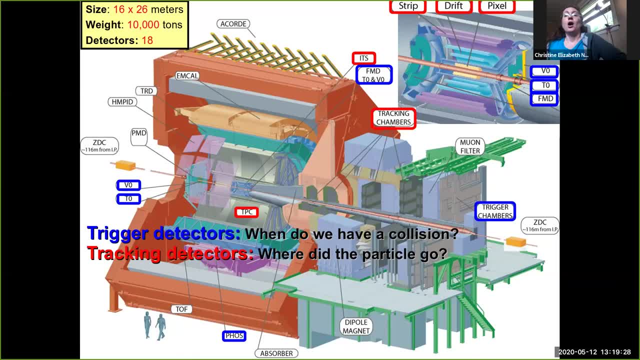 particles went as they came out from the collision. Almost all of these detectors work by looking at charged particles ionizing the detectors. So that means that a charged particle created in the collision comes out and as it moves through the detector it will knock electrons out of the material in the 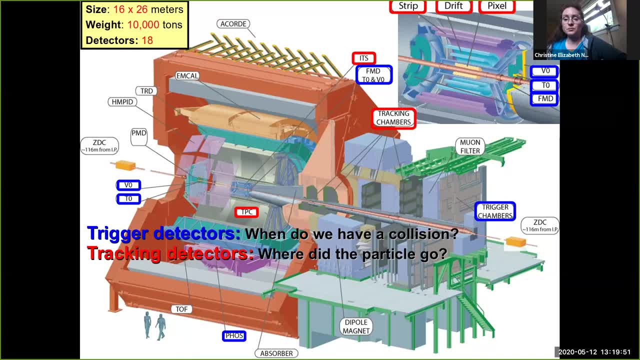 detector And then you use electric fields and you basically draw the charge out and you look at where the charge is, where the charge goes, to try to figure out where the track went. Most of these are so these are pretty much sensitive only to charged particles, because neutral particles are a lot harder to 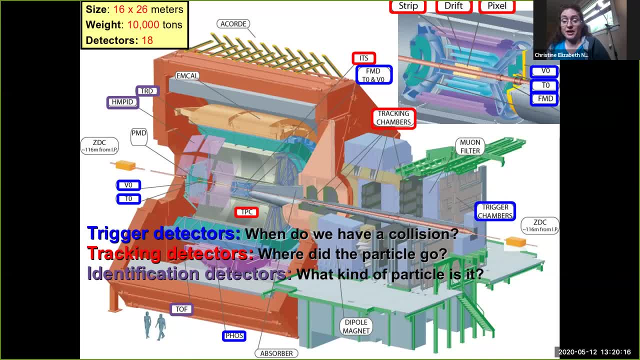 measure Particle identification detectors. they tell you what particles came out of the collision. and what particles came out of the collision, They tell you what kind of particle it is. Most of them work by telling you you do a simultaneous measurement of the momentum and the velocity and that gives you a. 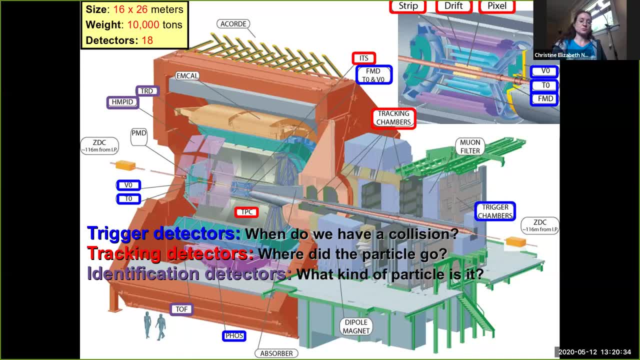 measurement of the mass so you know what kind of particle it is. And then you have calorimeters that tell you how much energy you have. So if I go with the camera analogy, the trigger detectors are sort of like the button you push to take. 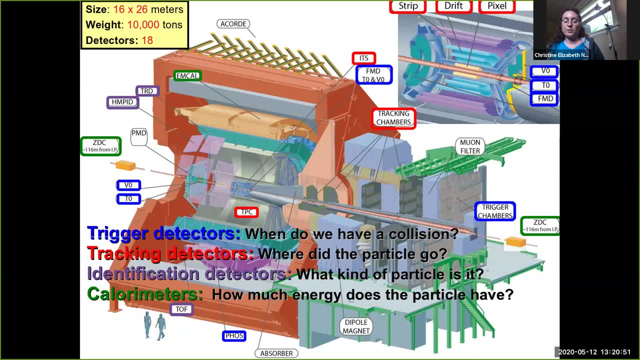 a picture. The tracking detectors give you a black and white picture, Particle identification detectors give you color and calorimeters give you maybe infrared as well. The details of every different detector vary, but they all, they all, most detectors can be classed into one of these different main types. And what you 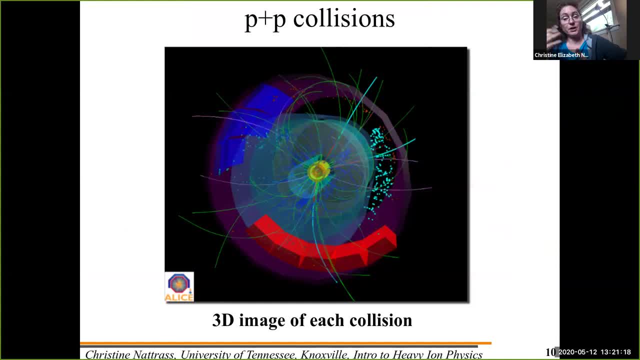 get now the. what you get out of this is something that looks like a picture of all of the particles coming out from the collision. So here you can see a proton-proton collision in the ELISE detector and what you see is the. the curved tracks are the trajectories of particles as they fly. 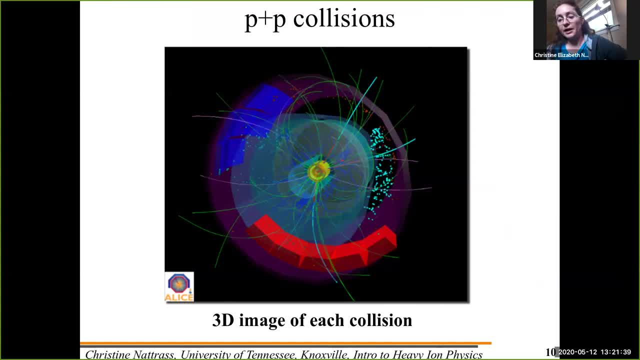 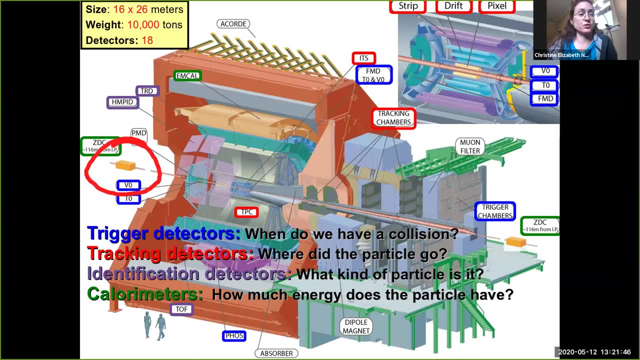 out. So what? I let me go back a bit In this. in this picture, what you see here is first of all the beamline. So the beamline is the trajectory of the particle. So the beamline comes right, goes straight through the detector. So this is where you 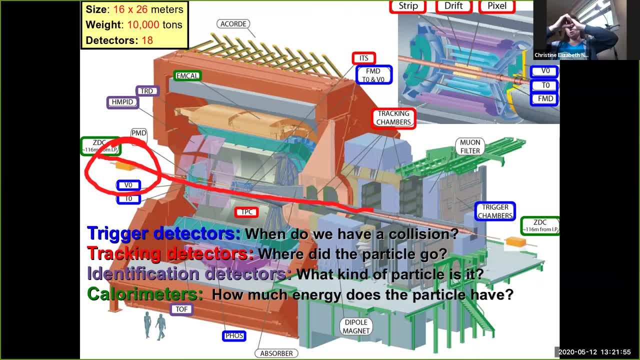 have one set of particles going in one direction and another set going in the other direction, And then you usually design the detector so that, when everything goes well, most of the collisions happen exactly in the center of the detector, where your detector works best, And then the entire thing is in an electric and a magnetic field. So this is where you 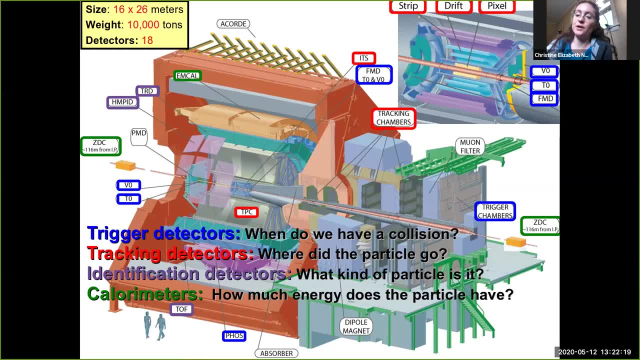 create. the went into a magnetic field to the center. So this is where it's between two field. So when you have a charged particle moving in a magnetic field, it's going to curve, just like you guys learned in freshman physics, and the radius of curvature is proportional to the momentum. And then you usually have 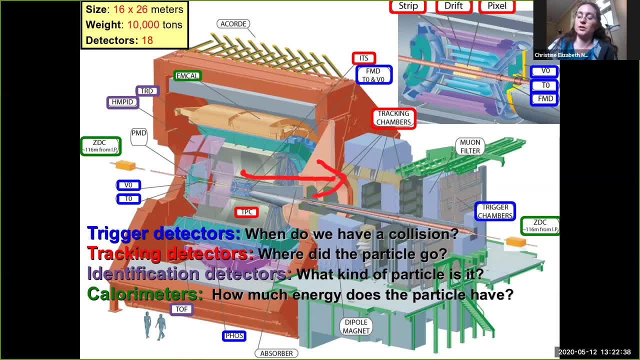 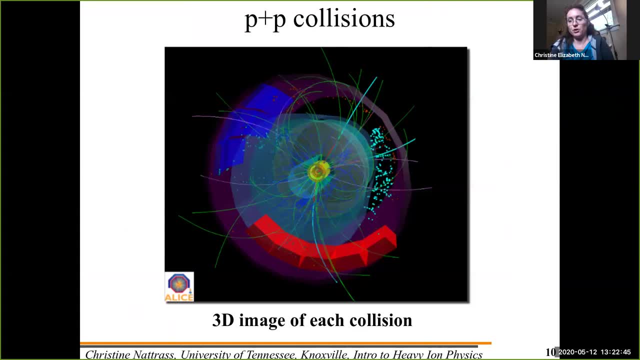 an electric field which draws those electrons coming out of the detector material towards the ends. So this is a proton-proton collision. What's been done here is that they've done something called tracking, So the raw data actually looks like a series of hits along one of these tracks, and then you have to have 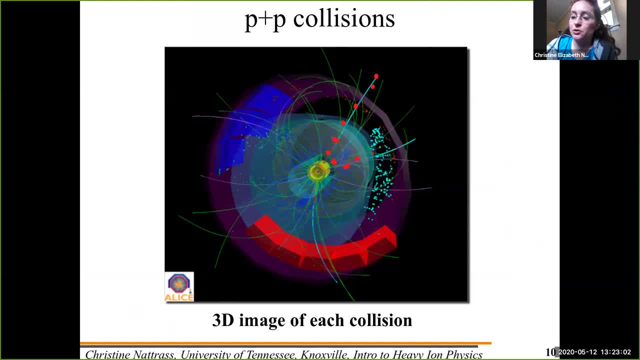 you have a set of software that tries to connect these so that you can tell where particles went, And that is a highly non-trivial problem. but mostly it's done centrally for the collaboration, So most of the time even grad students aren't worried. 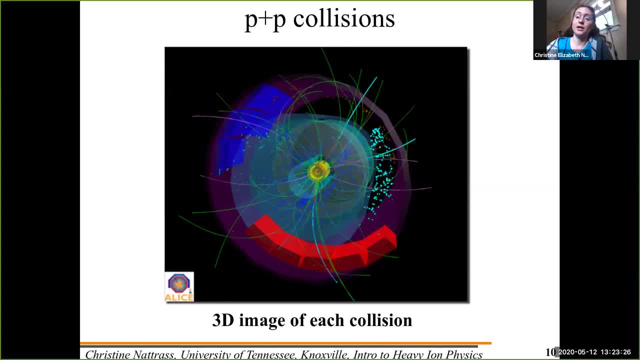 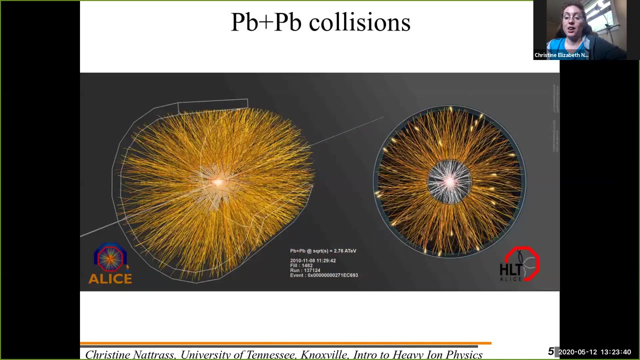 too much about those hits. They're using the final, the objects, where they're looking at the tracks themselves. And then this is an example of a heavy ion collision. So now you have a lot more particles. How many more depends on the collision energy and the system. but 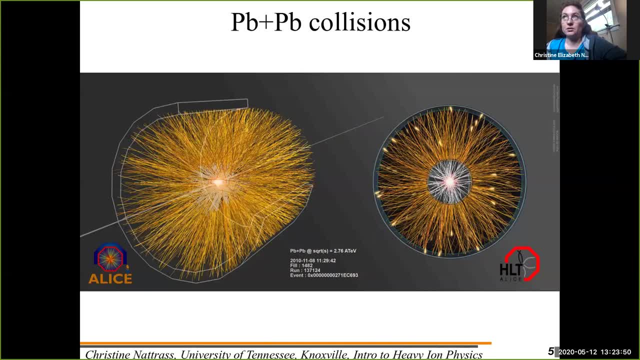 in lead-lead, it's the lead at LHC energies. it's something like 50 tracks in a typical proton-proton collision at most to something more like 2,000 tracks within the main part of the detector. So a lot of tracks, And I will pause there. 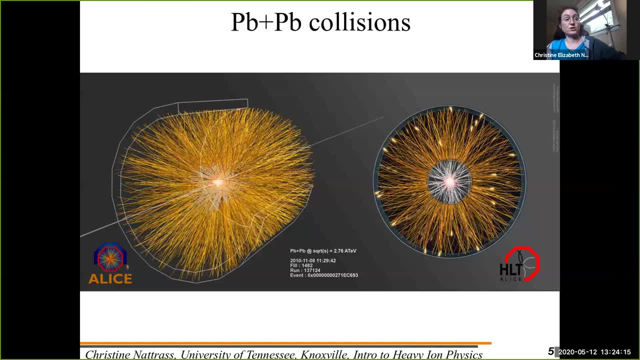 and see if anybody has questions on this. That was a big-picture overview, not a detailed overview of detectors. There's a lot more details. Who usually does the tracking? That's a good question. So these experiments, the smaller experiments that are active today, have still on the order of 500 people. So the labs. 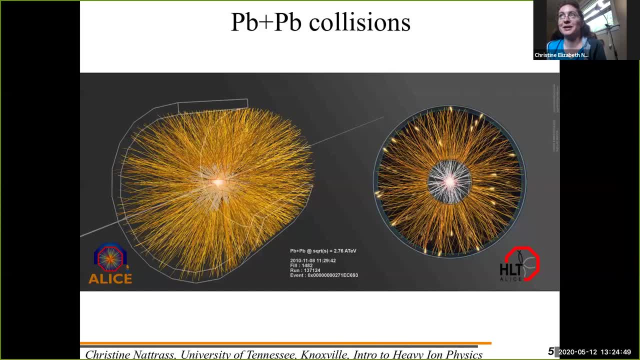 the bacteria in typically have a higher- over 1 million- Guru strata, So typically higher people who help with this. sometimes graduate students do get involved, but they're not starting from scratch and you start with software that worked before and then there is a central effort to do what we call reconstruction. 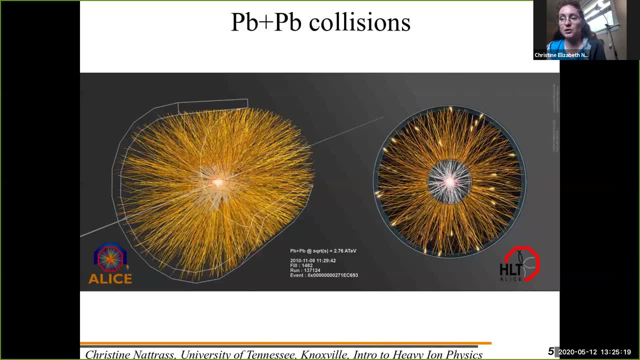 which is how you go from the raw data points to these tracks themselves. So typically you start on your own scratch slips and, again, no sixteen track assists. But so if anyone didn't get it text and with existing software and you're optimizing it and once it works, someone 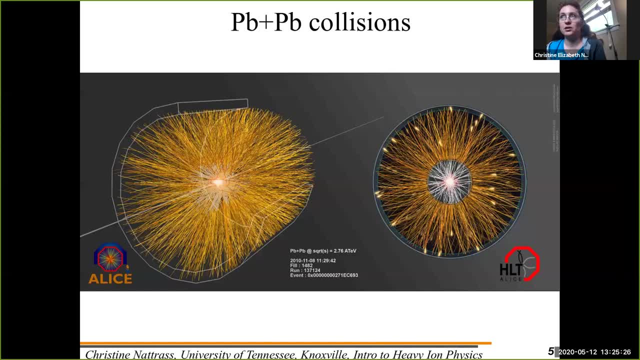 has to make sure that the reconstruction is done on all of the data, but it's not necessarily. how much effort that takes depends on where an experiment is in its life cycle. so at the beginning of an experiment there's usually a couple people working full-time to make sure that the tracking is doing what it's supposed to do, whereas at the end it may. 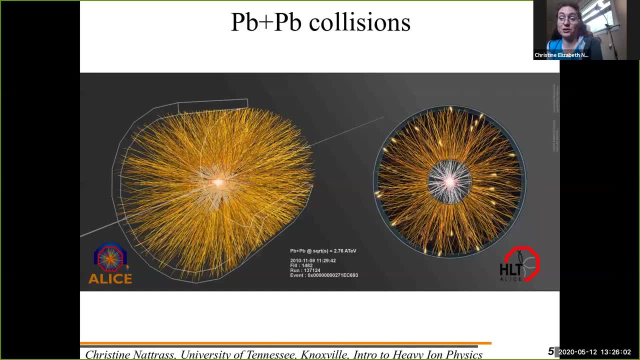 it may be a fraction of someone's time, because what they're really doing is making sure it's still doing what it's supposed to. there are a lot of. it also kind of depends on what your definition of doing the tracking is, because you do have people looking at quality assurance for each of the detectors and making sure that. 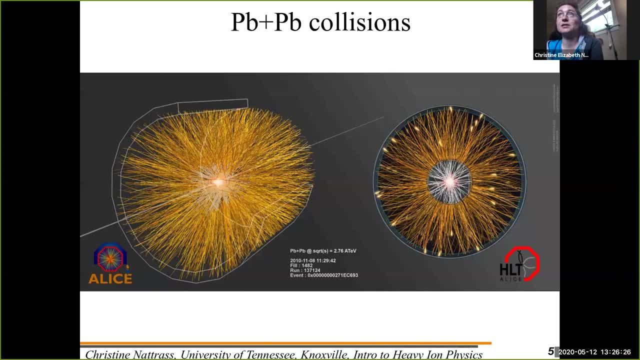 you. you have that, your tracks make sense. um so, for instance, on my last shift on the star experiment, the multiplicity went up, so something called space charge was a lot higher, which meant that you had a lot of ions in the detector. so the electric field was not what it was supposed to be. and when you looked at the 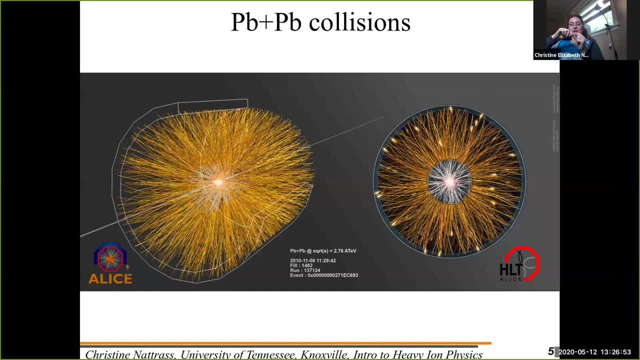 event displays. while we were taking data, the calibration tracks from lasers, which are supposed to be straight, were bent. so that tells you that a lot of corrections need to be done before you use that data, um, but it doesn't tell you what the problem is right away. so 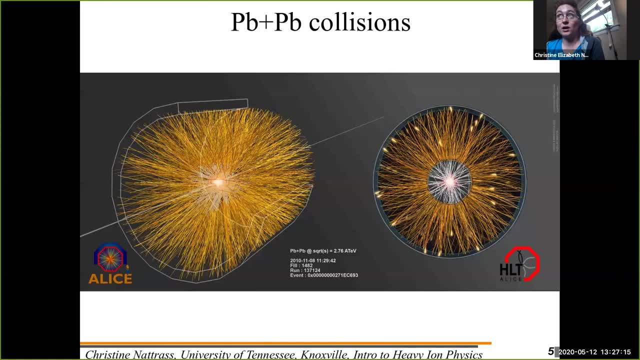 if you're doing qa quality assurance, that doesn't. I'm not sure that counts as tracking. um, it's usually a communal effort in general, um, so this question, let me so make sure that I can. the question was: I mentioned that a lot of gutenberg in e ghost route上面. 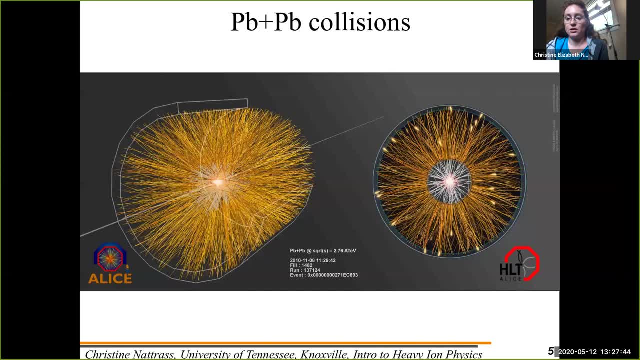 a xbox in e ghost route. 사 quel� mentioned that, if all goes well, collisions happen in the very center. Is this center region a few cubic centimeters? How much error can we have in defining this region? So this varies by the accelerator. So I'm going to share the whiteboard And I didn't 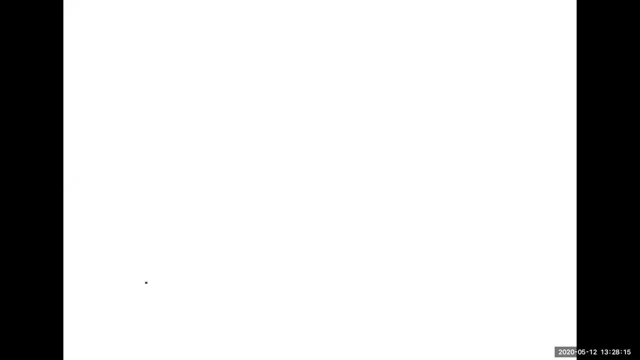 say anything about the accelerator, So, or the collider, So. in a collider you typically have two beams of particles, one going in opposite directions. So this is what it looks like in the big picture, But what's actually going on is that you have little tiny bunches like 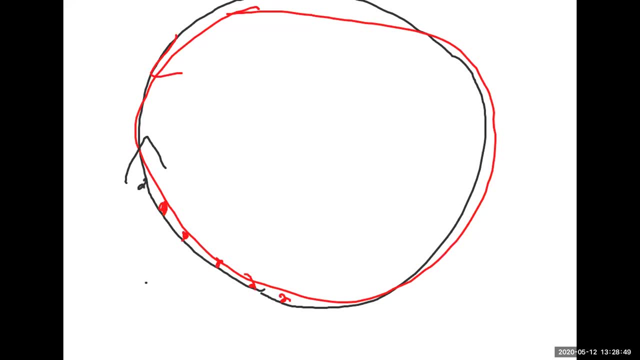 beads on a necklace And on the scale. when you're looking from the bottom down from an airplane, it looks like the beams are pretty much in the same spot, But if you look closer on the scale of the beam pipe, what you will see is that actually. 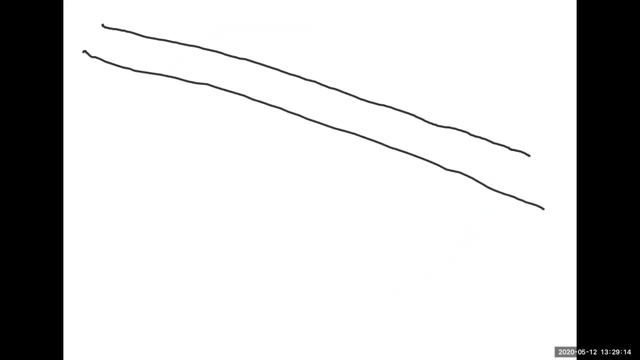 each of these beams. first of all, they have a finite width, So it's not. then, if you have a bunch of lead ions, They're not at 1.8, 0.7,, they're not solid and are not. falling off, as it will be if they fall off, or you finding out that the PILiest means like causes aA, I am not sure. So what leads us to that is the actual balance. the final balance will give paste of P2.. But that's. it's a lot better than nothing. So each beam is. 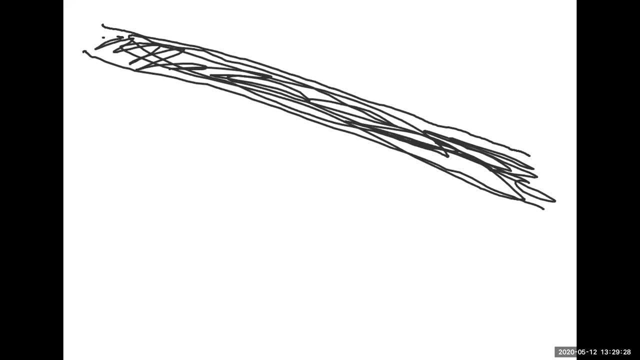 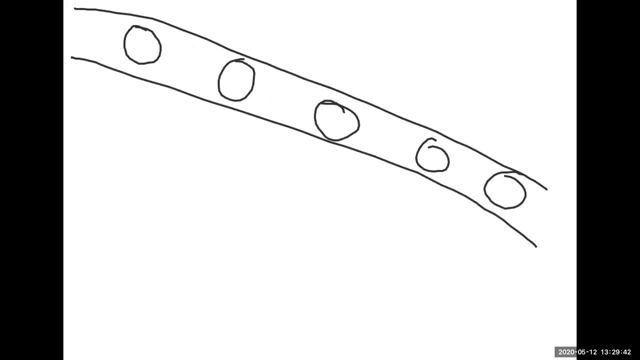 They're not at one little tiny point, but you have the direction. Actually, let me draw it a little bit differently. So you have sort of a track that they will follow, and inside you have bunches, And the other beam has bunches too. 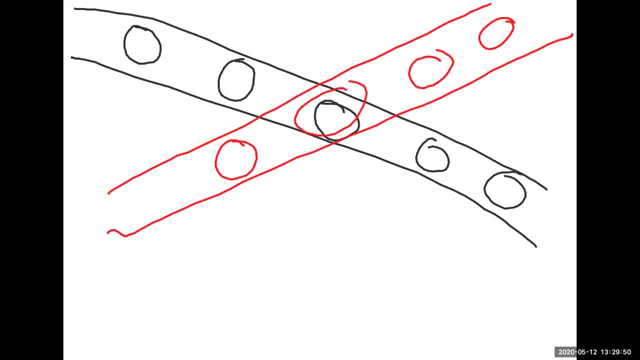 And then you can only have collisions where these two bunches cross, And this is called the interaction diamond, And at the Large Hadron Collider that interaction diamond is plus or minus about 10 centimeters, So the whole thing's about 20 centimeters from the center of the detector. And then at the Relativistic Heavy Ion Collider. they've worked on trying to. I believe the design spec was the same as the Large Hadron Collider, but the actual interaction diamond was more like 60 centimeters and they've worked on making it smaller. 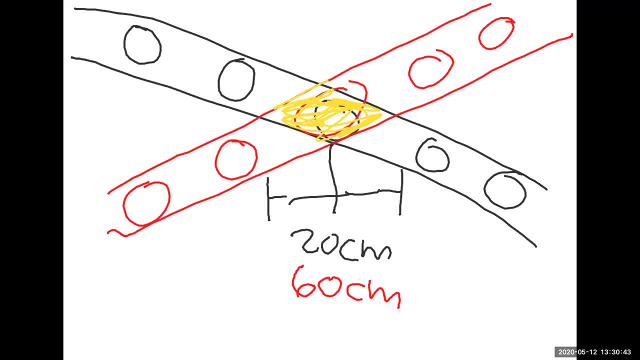 I'm not sure what the latest was, what the best they could do was, But this is also a statistical, So for any given collision it's going to happen at one spot here, so one spot around the detector, And you actually can get some because you have a statistical distribution of where the ions are in the bunch. 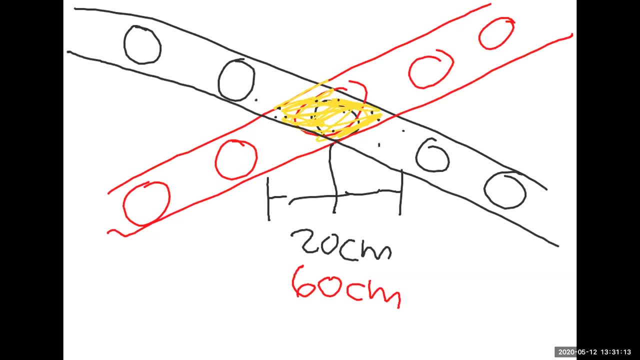 So you can get some collisions that happen slightly outside of that interaction diamond. Let me go back to the chat and make sure that I So we usually don't talk about it in terms of cubic centimeters. The relevant distance is the length of that interaction diamond along the beam pipe. 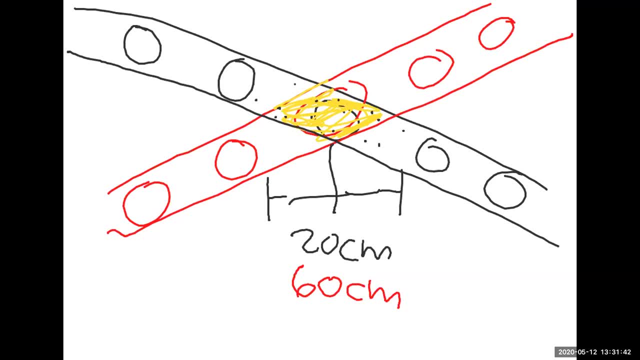 Usually the beams are. The beam pipe is on the order of centimeters, depending which collider you're talking about. So the beam pipe is on the order of centimeters, depending which collider you're talking about, And then the width of the beam is also on the order of a centimeter or two. 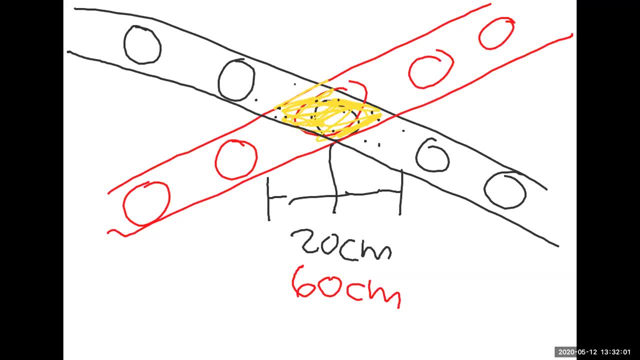 The diameter is like a centimeter or two. You actually do. There's a lot of cool details about this as well. So at the Large Hadron Collider the Elise detector is slower than ATLAS or CMS, So they actually make the bunches larger in the 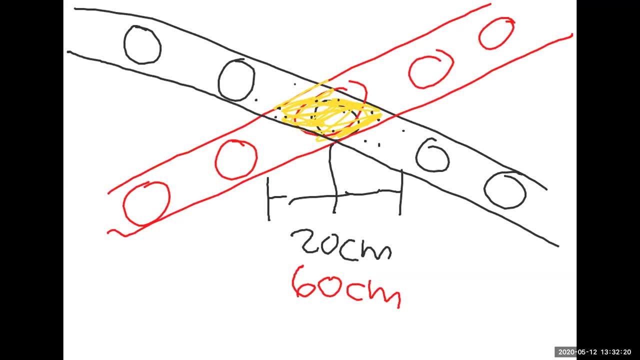 The ALICE interaction region so that you have a lower collision rate. But at ATLAS and CMS they squeeze the bunch down to have the smallest diameter they can so that you get the highest collision rate possible. There was a question: how do you accelerate them to the speed of light, or at least close to that? 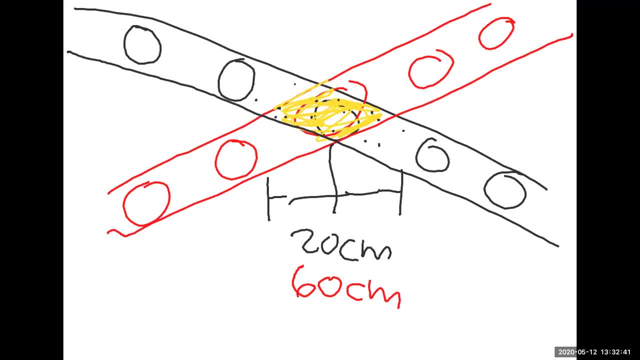 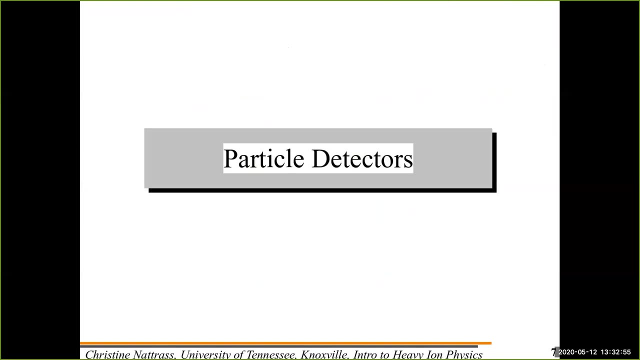 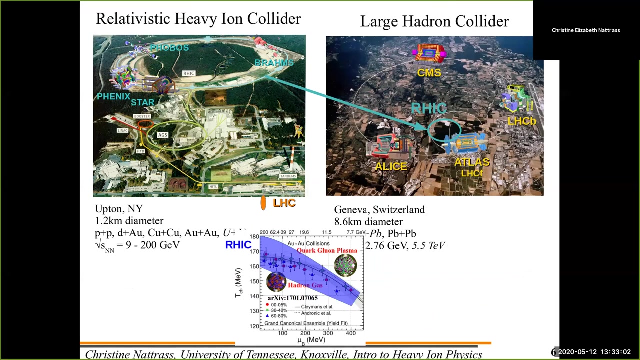 In a lot of very slow stages. So here I'm going to go back to The slide I had of the colliders, because what you see is a bunch of different accelerators And on the fly I'm going to remember all of the names incorrectly. 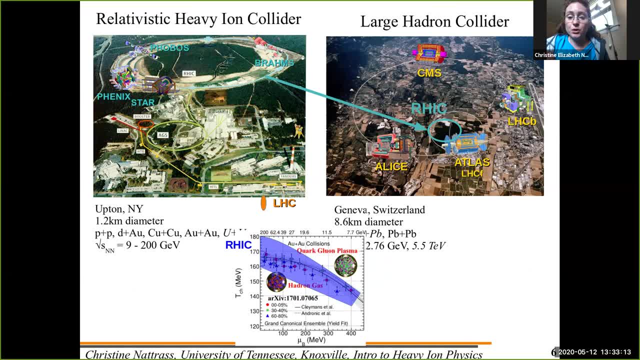 so I'm going to just avoid mentioning them by name. But both the Large Hadron Collider And the Relativistic Heavy Ion Collider have these. You start with some ions that have just a few electrons stripped out of them, And when you do that, you can accelerate them in a tandem accelerator. 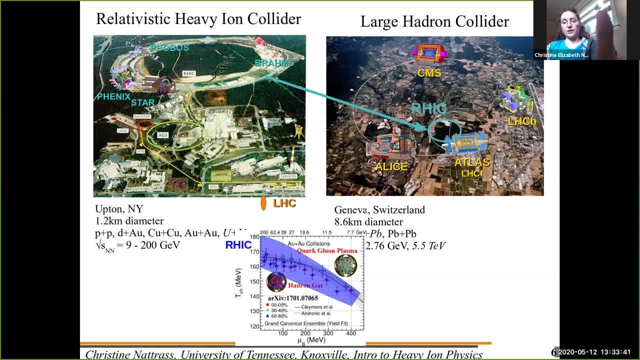 so that just by using an electric field you get them going faster. And then You have a few different stages, so they start out fairly slow And you send them through a foil so that it strips more and more electrons off of them. 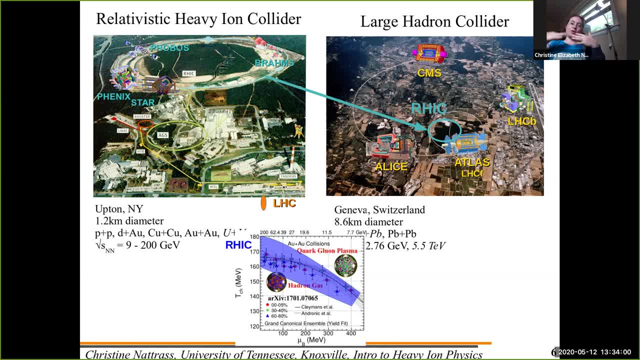 At that point because you have a sample of ions. you actually have a mixture of different charge states, So you send them through. Let's see if I can. I've lost my ability to mark up on this screen- But you send them through another accelerator. 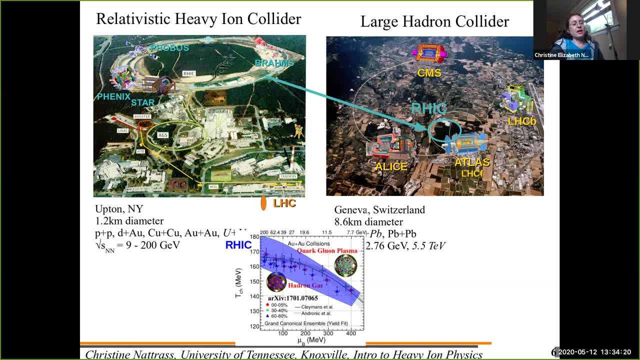 so you send them through a turn with a magnetic field and that lets you select the charge state so that you're sure which charge state you have, And then you send them into a smaller Well, a larger accelerator and then another larger accelerator. 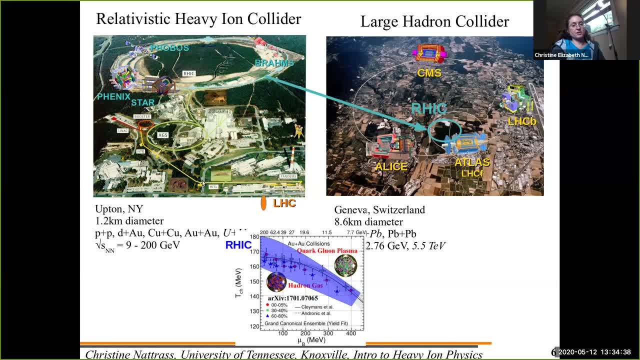 So at RIC it's a tandem accelerator which is basically just a giant that you send them through an electric field And followed by a booster accelerator and then the alternating gradient synchrotron And then finally they're injected into the relativistic heavy ion collider. 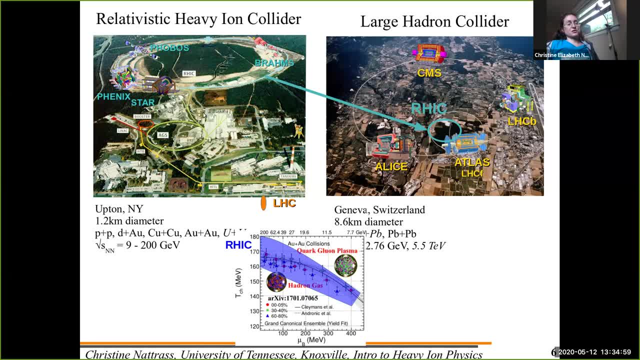 And at each of these stages- actually it's a clever trick They are using- Once you get into the relativistic heavy ion collider, you're actually using electromagnetic radiation to accelerate them So that When you, When you have, When you have an electric field, 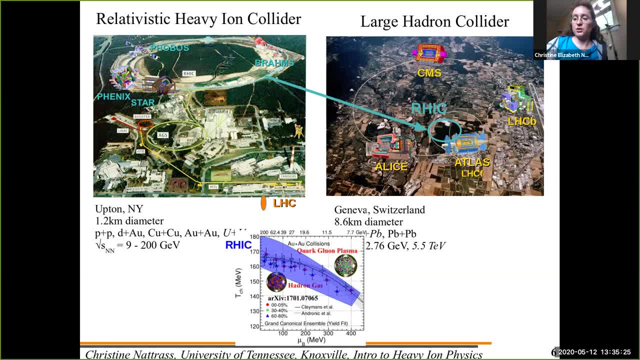 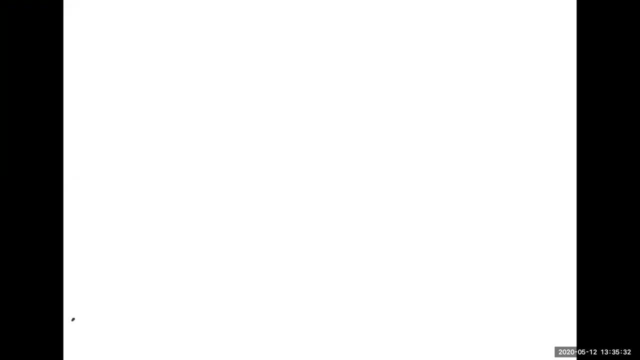 When you have electromagnetic radiation, you have, You have an electric field that varies with space and it will accelerate. So if you have a bunch of, If you have a bunch of ions in here, it will accelerate the slower ions. Let me actually try to draw this a little bit. 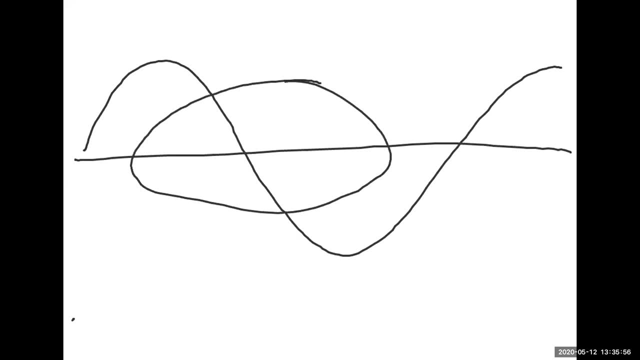 So it's got some dimensions. So the electric field actually works to accelerate the slower ions and decelerate the faster ions so that you get a focusing effect from the electromagnetic radiation And you just slowly change that- The, The radiation and the magnetic field- to slowly bring it up to the right speed. 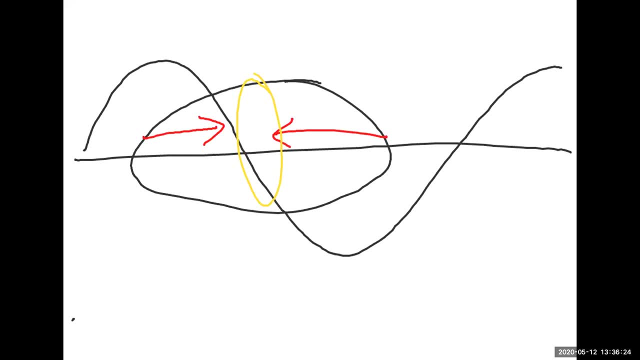 to the speed you're at, Although at those speeds you usually quantify it in terms of, not the speed, but in terms of gamma, Because the The speeds are so close to the speed of light that it's not convenient to use the speed itself. 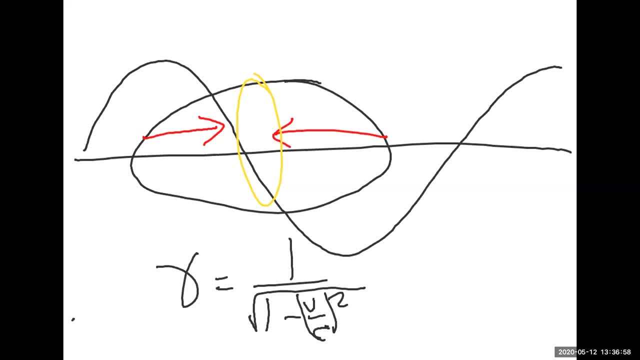 And then Let's see. So I think that answers the questions. If I don't see other questions, then I'm gonna: Ah, Do you? Do you use the tracks to reconstruct jets, or how do you relate tracks to primary particles? 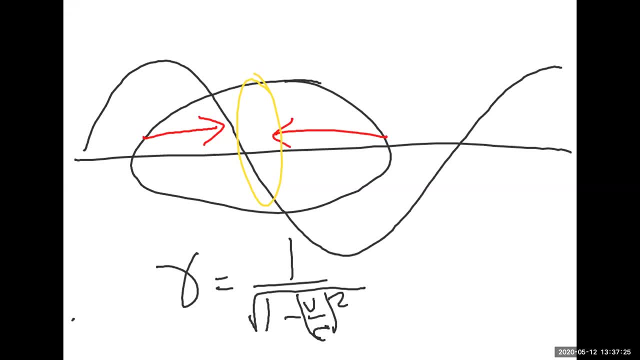 I am going to come back to jets, because jets are a whole different can of worms. I have two different sections on jets. The question of how you relate the tracks to primary particles is a really good one, So I am going to. 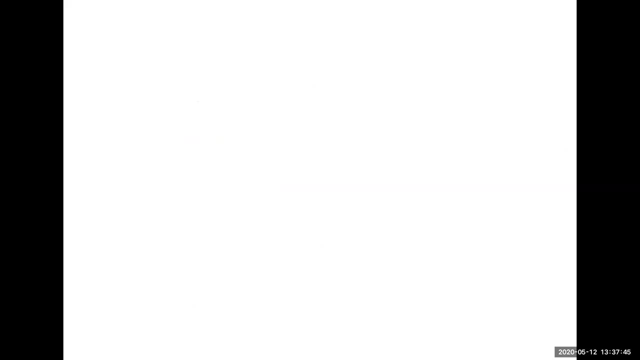 So what your raw data look like. So here's the beam pipe and then here's your detector, And so we're looking at the beam coming in and out of the board here And your raw data are actually hits, and so if you have, 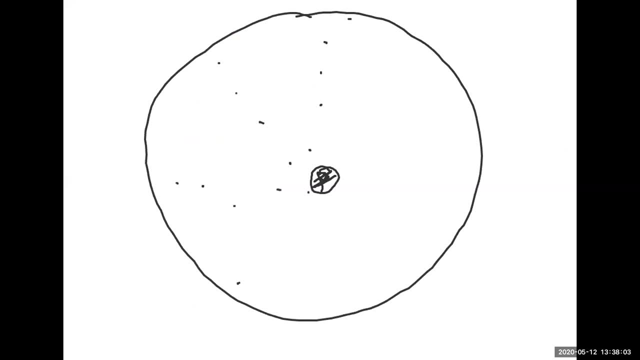 So you have little points along the track. If you have only a few points, it is not too hard to draw a line between them and say this is my track. What you usually do is you actually start from the outer edge where the hit density is. 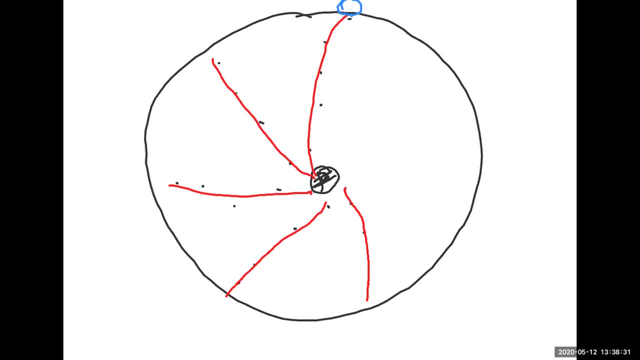 lower and you basically try to inch your way all the way in, And there is an assumption that one of those tracks- something that is basically a continuous line is probably- probably corresponds to what was left by a single particle, And the ambiguities in that are. 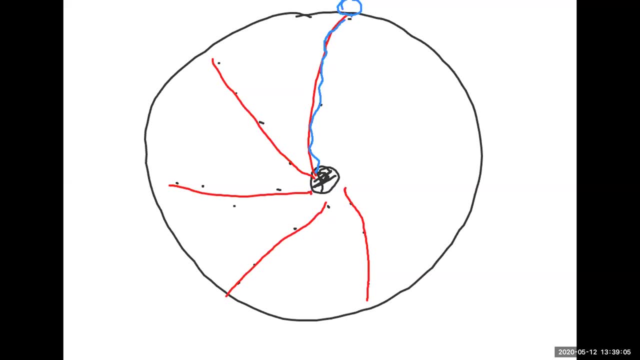 basically what comprise a lot of the systematic uncertainties in the measurement. So what we can do is that we simulate the detector and we simulate what happens when you have a charged particle going through the material of your detector and you can say: 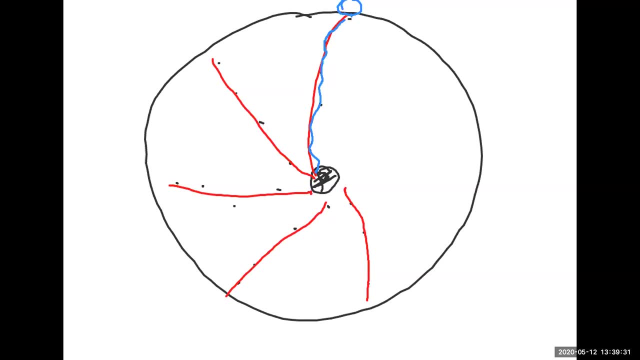 okay, when I have a pion, a positively charged pion, going through my detector, it leaves this many tracks and this is how it behaves. and you test your software for reconstructing tracks on those simulations And you can also do things like: 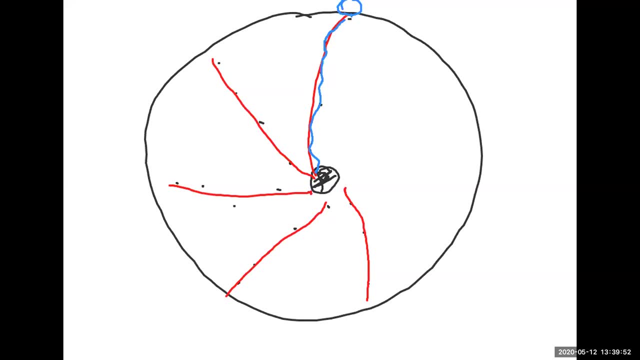 put parts of your detector in a test beam where you know the energy and the particle type of the particles that your detector is getting hit with and you can make sure that it behaves the way that you think that it should. And most of the time, 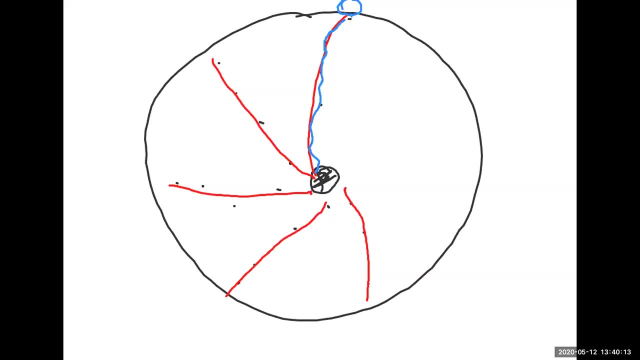 in a typical analysis that gets published, you have a lot of hits along that line. So in the ELISE detector you have, if a track goes through the time projection, the time projection chamber, which is the main tracking detector. you have 135 points along that track. 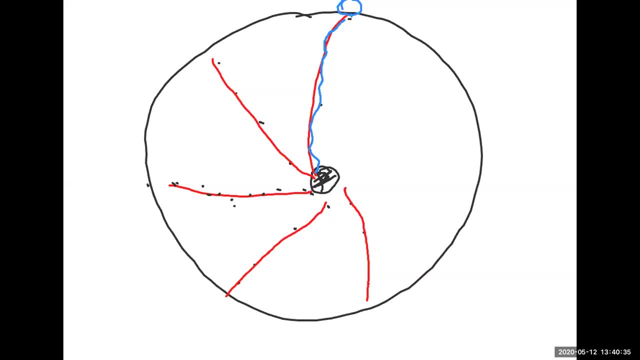 So, and you require: for a good track, you require something like 80% of the possible hits. And then there's other detectors, that called the inner tracking system, that give you another six hits. But there is an assumption there that if you can form a continuous line, 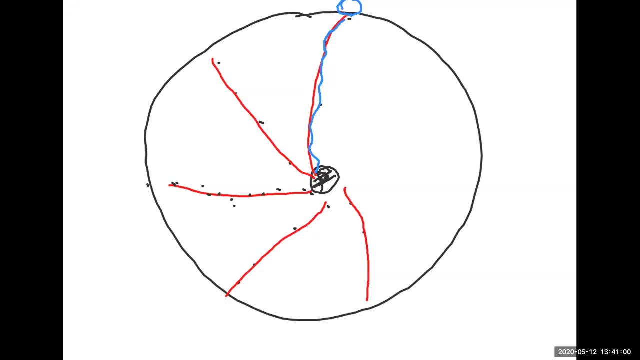 that it comes from one particle. This is why we do. we have a bunch of quality assurance cuts. So when you fit the track to a line where you assume that the line is curving in a trajectory to match the magnetic field, you 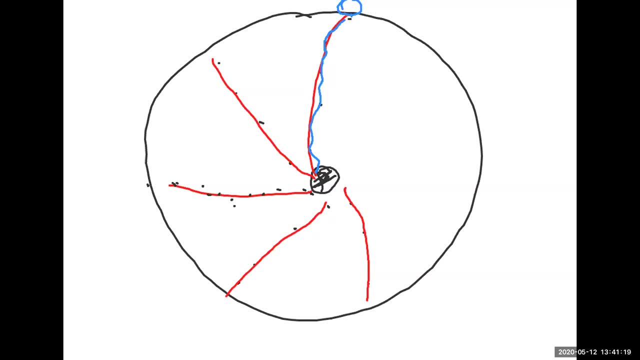 you get a chi-squared on the track. chi-squared is actually- let me do a new sheet- Chi-squared is the value, the sum over the number of points of the value you observe minus the value you predict. quantity squared. 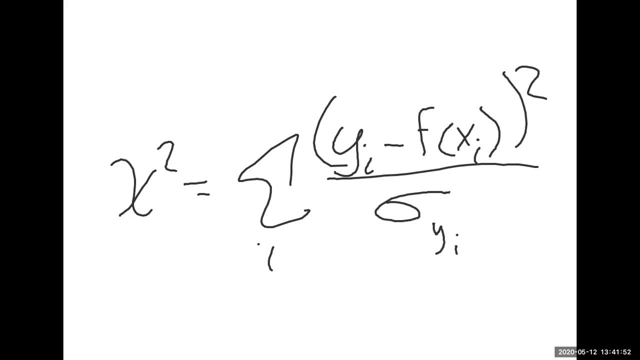 divided by the uncertainty. So you get this chi-squared and that gives you a measure of the quality of the track And there are a number of ways that you can throw out things you think are bad tracks, which is an imperfect process. 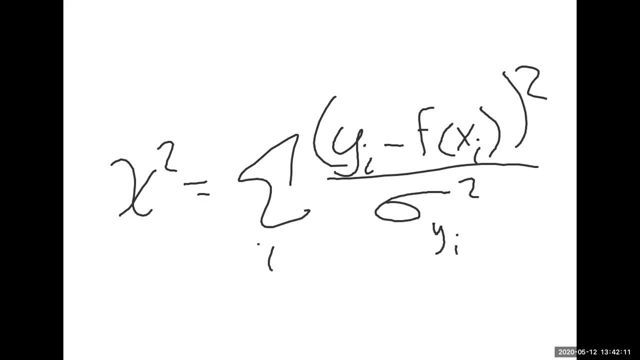 So, depending on your detector, you usually throw out good tracks erroneously, and sometimes you have bad tracks erroneously And the devil is in the details. So that's a very good question: Are there situations where there are several tracks near each other? 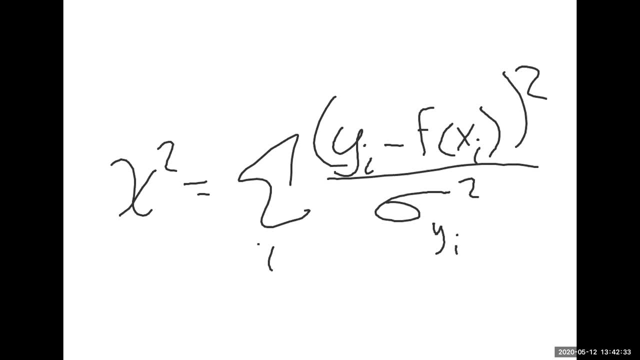 from one primary particle. I think that what you're talking about is that I actually have one real particle, but I have erroneously reconstructed it as two, So something like that. Yes, that happens Most of the time, so you have different ways. 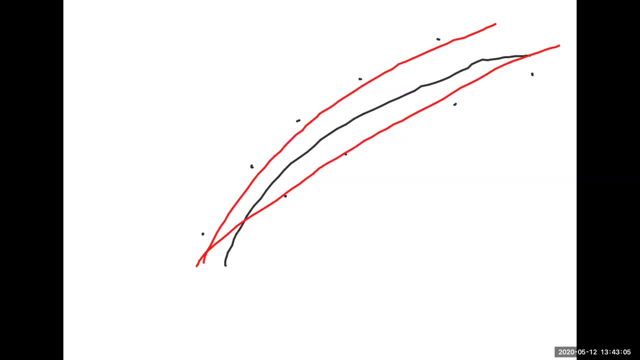 that the tracking, the trackers, can work. Often you let you insist that you require that each hit is associated with one track, and it is usually associated with the track where it is which it is closest to. And if you do that, 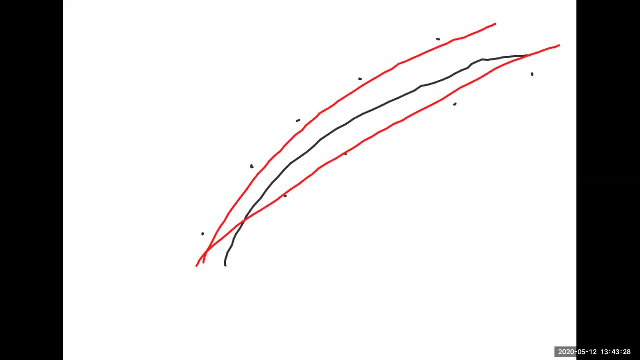 then in this case, where you get two tracks from the same particle, neither of those tracks- well, in this case that I drew, each of those tracks has about half the number of possible hits. So in the ELISE detector if you have 135 possible hits, 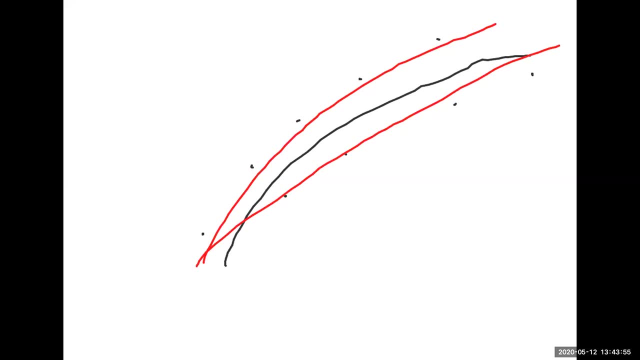 you know, one of the tracks might have 70 hits and the other has 60, and then some of the other hits went somewhere else because they didn't get associated. So usually your track quality cuts would cut that out and so that track would not enter your sample. 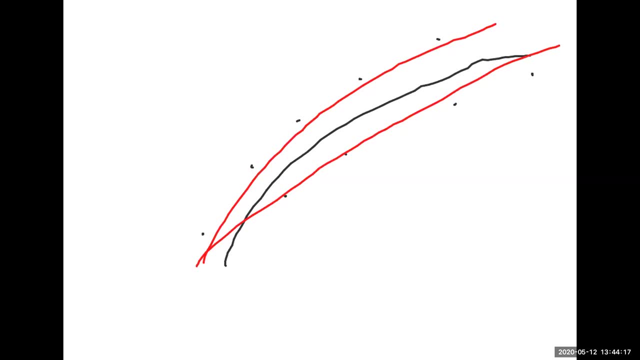 That also means that you then would not have reconstructed this particle. There can be cases where you have- you know here's your particle and the hits that it actually left. maybe your particle does something where it then hits detector material and it is deflected. 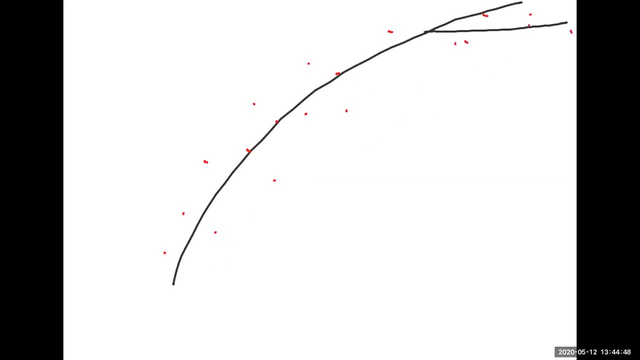 and then you suddenly have. you have hits, but they don't all line up along the expected trajectory. So then you could reconstruct it as this track and a shorter track. This shorter track is not going to have very many hits and it's not going to start near. 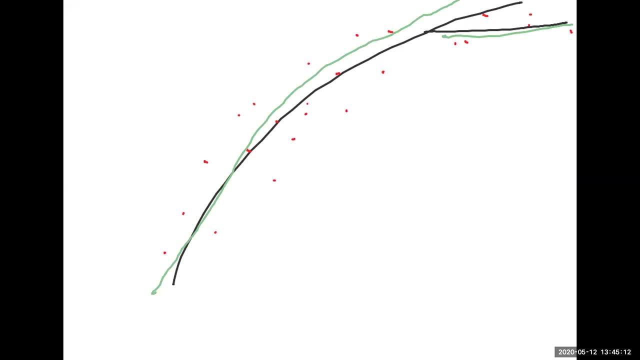 the primary vertex, So most analyses would actually not use it, So if I go back here. So another cut that you usually do to make sure that you have good tracks is that you require that your track is close to the primary vertex. 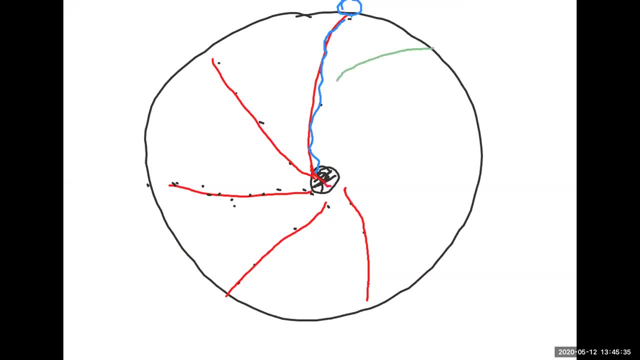 So if you have a track hanging out over here, you would not use it in your analysis. There are analyses where you're trying to analyze those tracks because you're looking at things that can create shorter states. So if you have stub tracks like that,